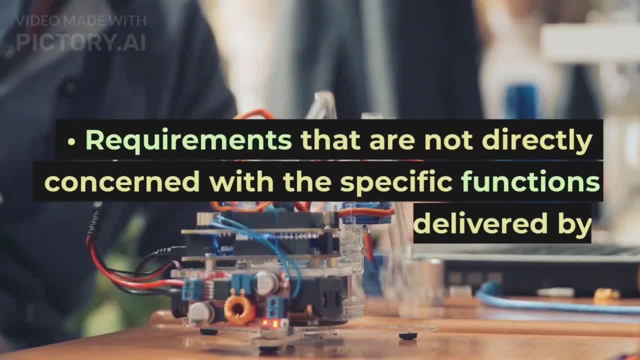 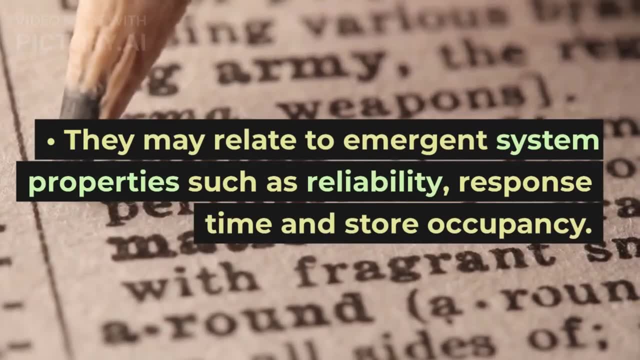 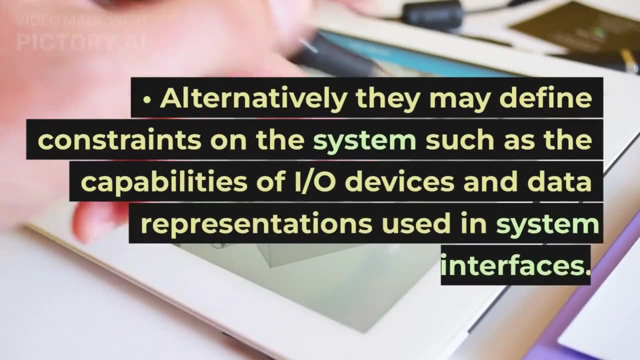 Non-functional requirements: Requirements that are not directly concerned with the specific functions delivered by the system. They may relate to emergent system properties, such as reliability, response time and store occupancy. Alternatively, they may define constraints on the system, such as the capabilities of IO devices and data representations used in system interfaces. 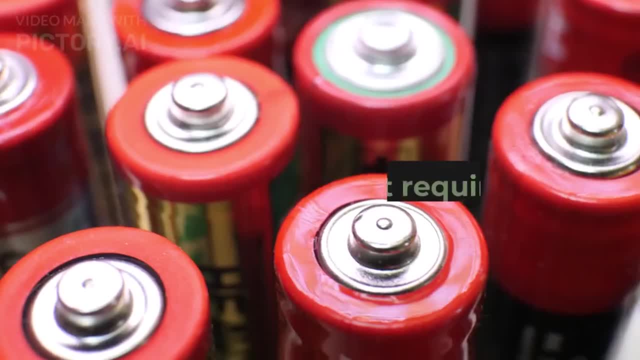 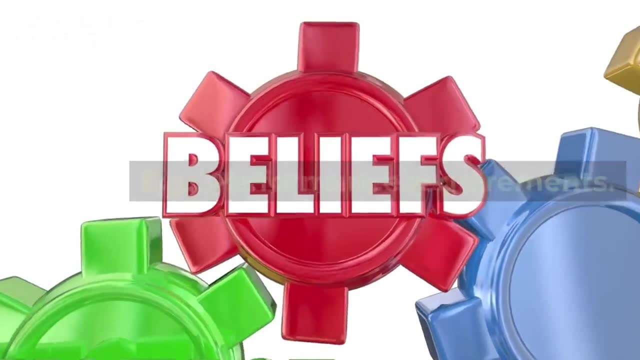 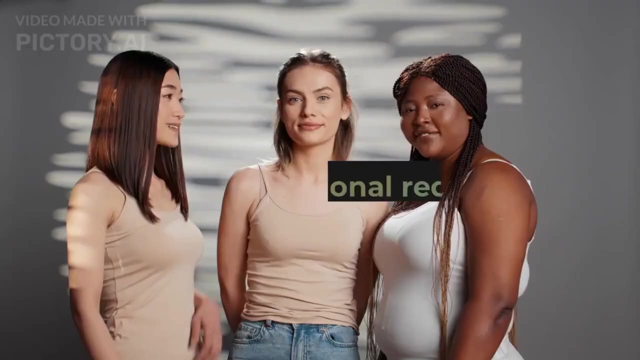 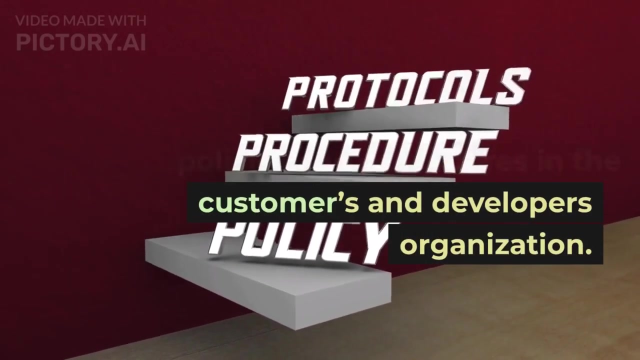 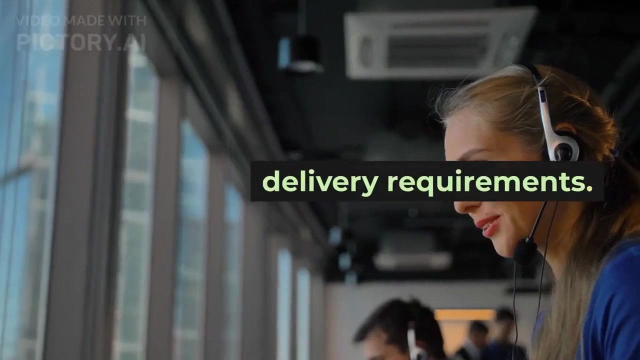 Types of non-functional requirements. 1. Product requirements: These requirements specify product behavior, eg performance requirements, reliability requirements, portability requirements, usability requirements. 2. Organizational requirements: These requirements are derived from policies and procedures in the customer's and developer's organization, eg process stands, implementation requirements, delivery requirements, 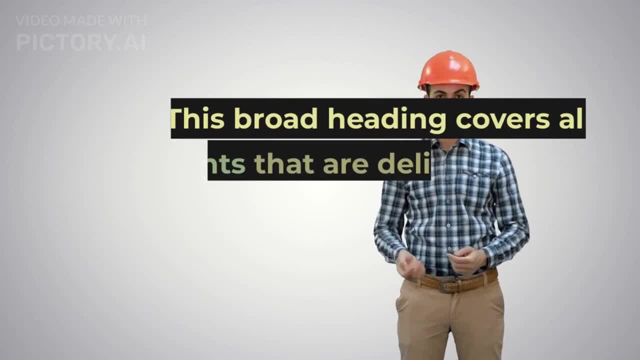 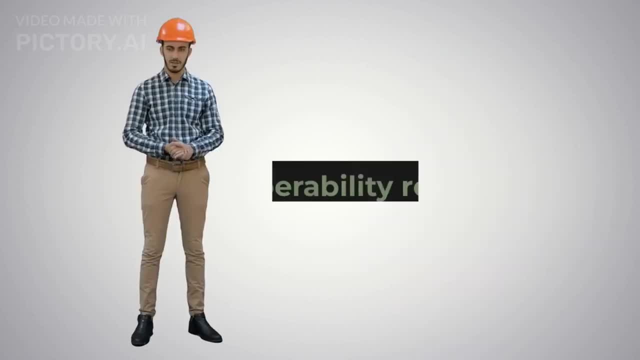 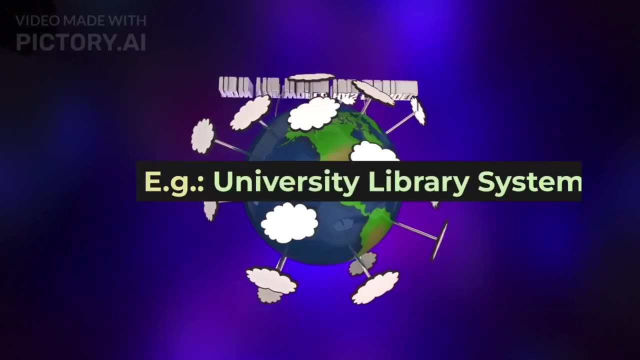 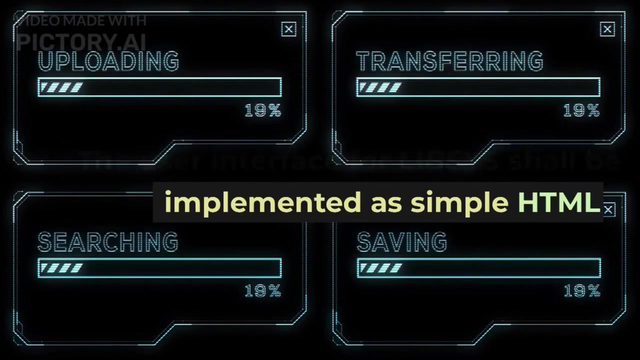 3. External requirements. This broad heading covers all requirements that are delivered from factors external to the system and its development process, eg. interoperability requirements, Legislative requirements, Ethical requirements- eg. University library system Product requirement. The user interface for Libsys shall be implemented as simple HTML without frames or Java applets. 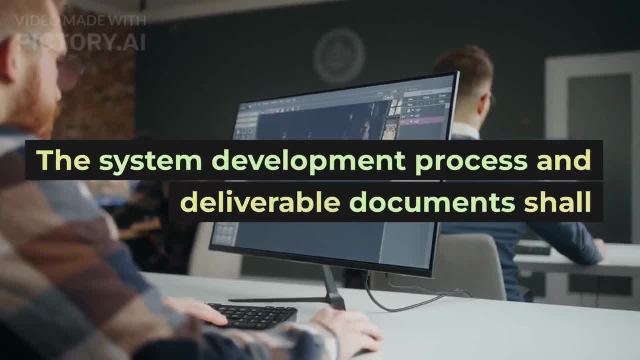 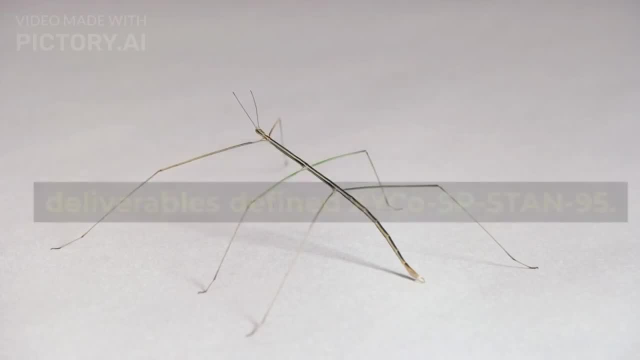 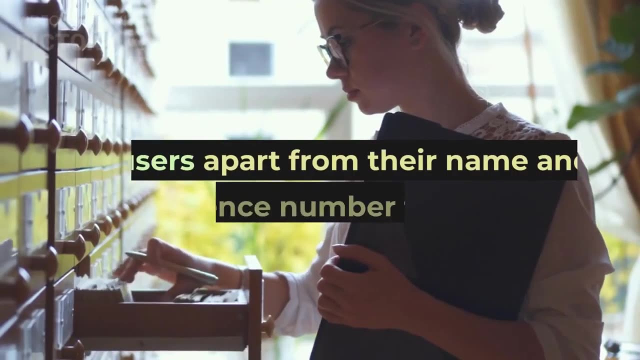 Organizational requirement: The system development process and deliverable documents shall conform to the process and deliverables defined. XYCoSP, Stan 95.. External requirement: The system shall not disclose any personnel information about system users apart from their name and library requirements że we need to healed. you never come over to the library. we call some contacts which you значит a binding you. you can view your library for a freeLEY you for reference number to, frankly, the library staff. 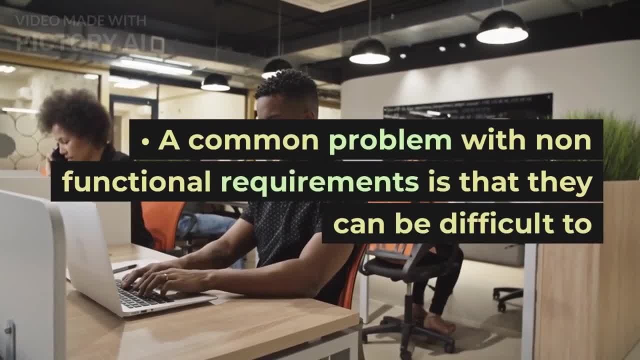 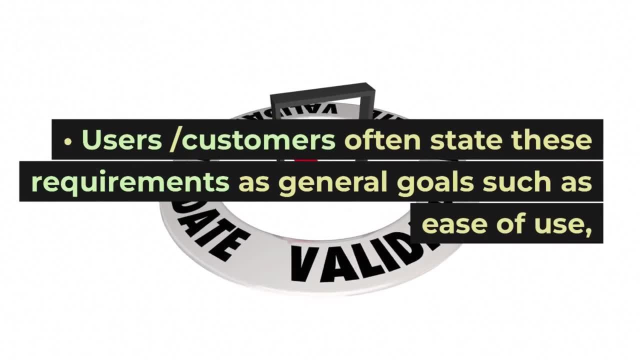 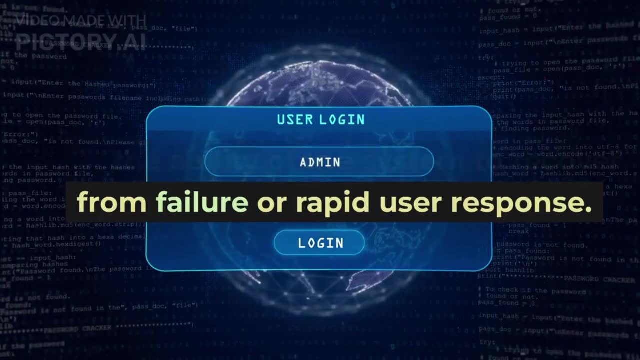 we can come identity common problem makes a common problem with non functional require is that they can be difficult to verify. users slash 들어가. Stephen state these requirements of either old, the ability of the system to recover, to recover from total. whenever possible you should write non functional requirements quantitatively. 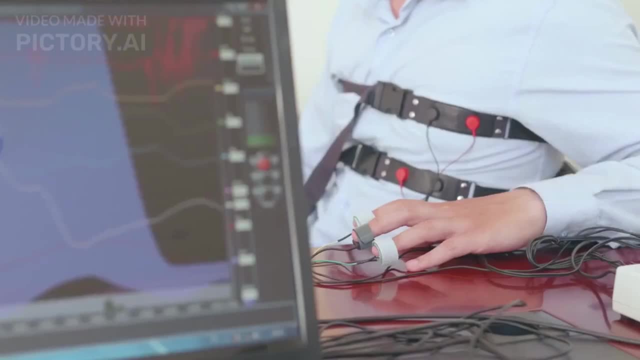 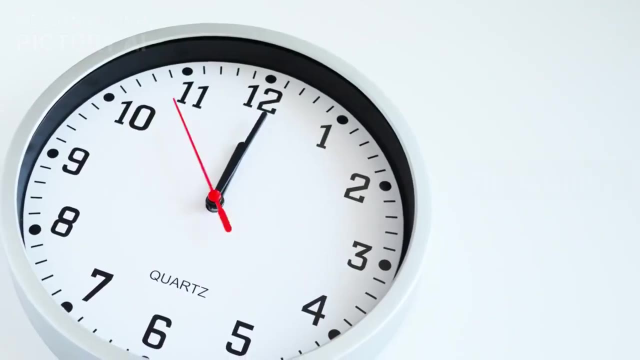 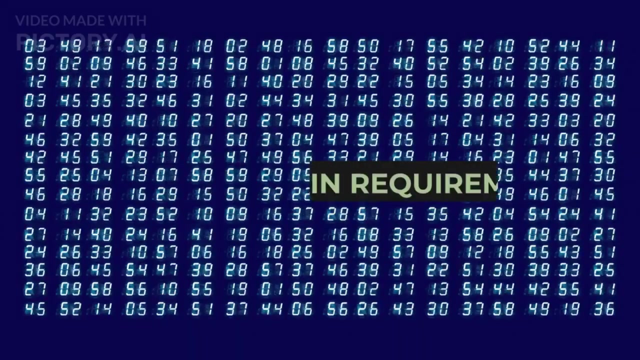 so they can be quantitatively tested: speed processed transactions: seconds. size, k bytes. ease of use, training time, reliability, rate of failure occurrence robustness, time to start after failure, portability, number of target systems. Domain requirements: Domain requirements are delivered from the application domain of the.